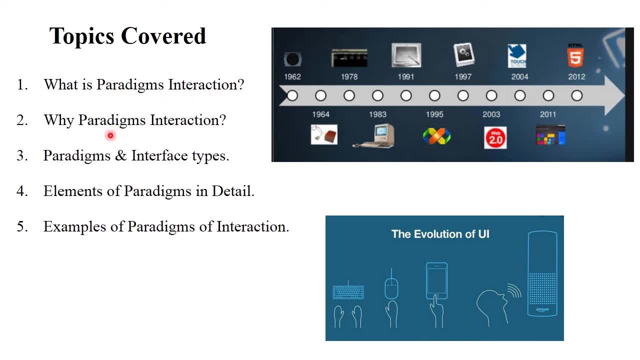 What is Paradigms of Interaction? Why Paradigms of Interaction, Paradigms and Interface, Type Elements of Paradigms in Detail and Examples of Paradigms of Interaction. So let's see one by one, First what is meant by Paradigms. 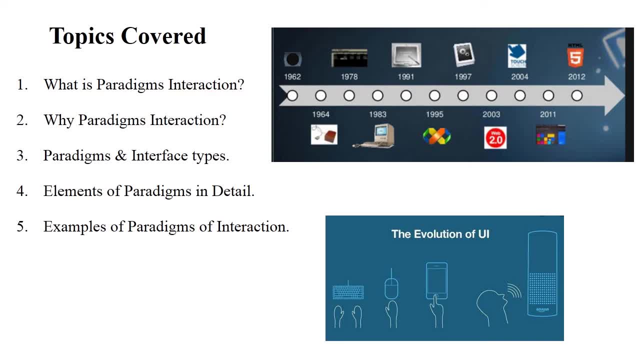 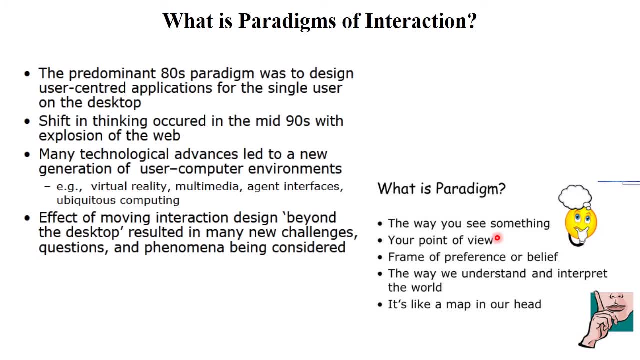 Paradigms of Interaction Next. So Paradigms of Interaction, It simply means the way you see something, Your point of view regarding the latest technologies, regarding latest inventions, etc. So Paradigms, or Predominant 80s Paradigms, is way to design a user centered application for the single user on the desktop. 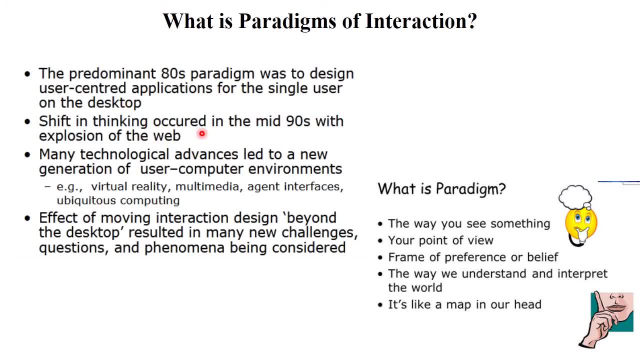 Right. But in 19th century shift is thinking occurred in the mid of 90s, explosion of the vape. Many technological advance like new generations of user computers, environments like virtual reality, multimedia agent, interface, ubiquitous computing, these all kind of applications or new inventions are generated. 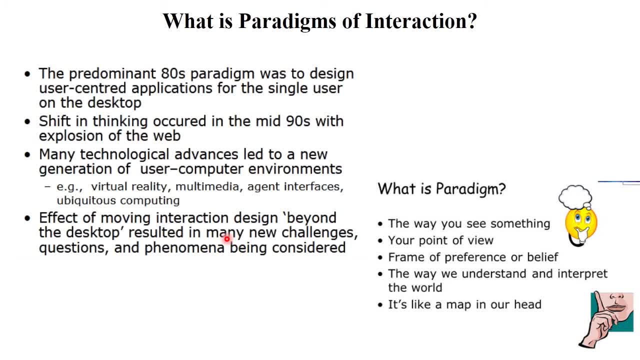 So effects of moving interaction design beyond the desktop is resulted in many new challenges, questions, phenomena is being considered Right. So history or study of all those things as per their generations or as per their centuries, from 80s to 21st century, 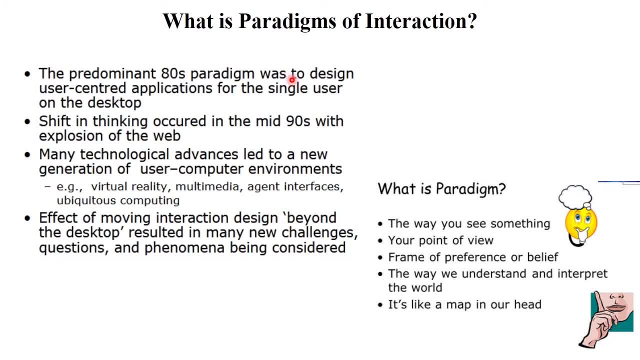 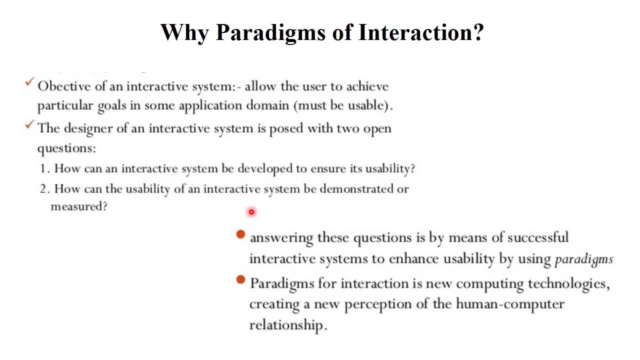 Right To study of all those things is called as Paradigms of Interaction, Clear. Next The next: Why Paradigms of Interaction? Why we study all those things. So the objective of interaction system. it allow the user to achieve a particular goal in some application. 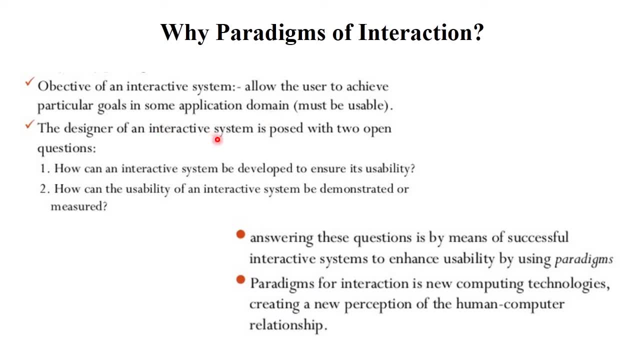 Right. So designer of interactive system is posed with. there are two most important questions. The first question is: how can an interactive system be developed to ensure its usability? We already learn usability is one of the most important goal of the technologies, of the applications, etc. 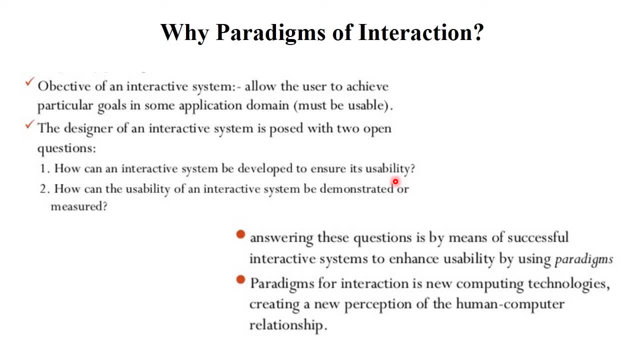 Usability means easy to use, easy to learn, Right. So and next question is: how can the usability of interactive system be developed, Right? How can the usability of interactive system be demonstrated or be measured? So, answers of all those questions: by means of successful interaction system to enhance the usability by using different paradigms. 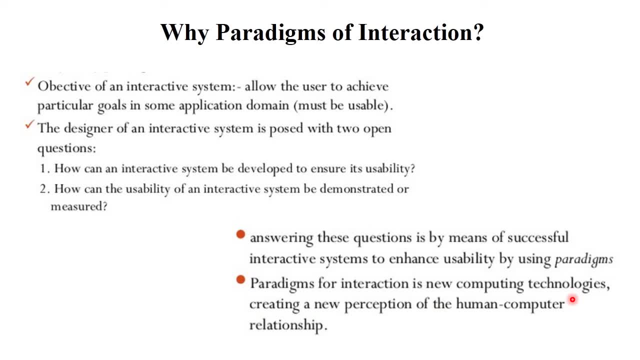 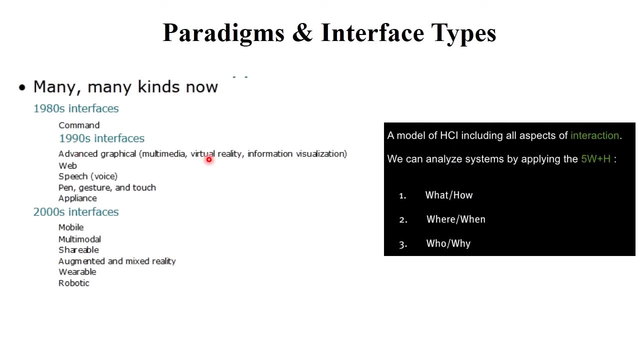 So Paradigms of Interaction is a new computing technologies. It creating a new perception of the human computer relationship, Right, So that's why we studied Paradigms of Interaction Clear Next. So Before start, the elements of Paradigms. 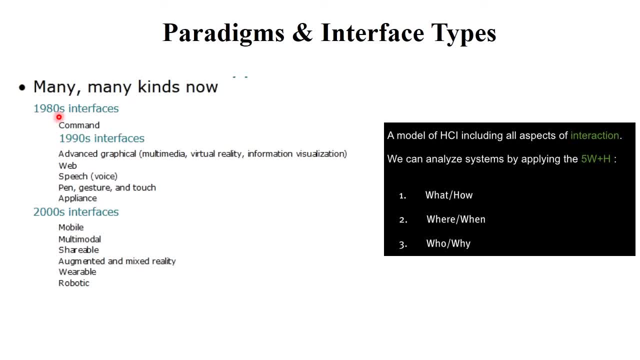 See here. These are the generations. Like in 1980s, interface includes command line interface. In 1990s there was advanced graphical, like multimedia, virtual media information visualization, Then a web speech pen gesture appliances And in 2000 interfaces was invented like mobile, multi model, shareable devices, augmented and mixed reality. 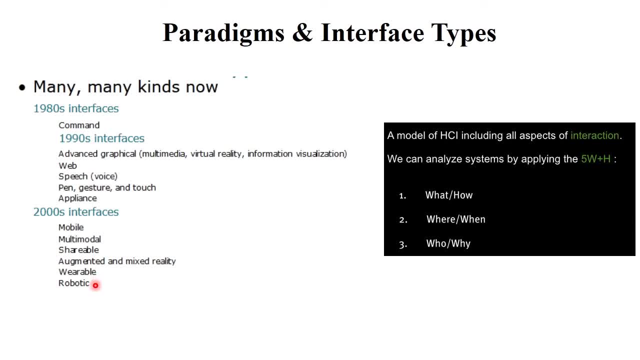 There are, wearable devices are also present And robotics- Right. So these are the inventions or these are the generations, A model of human computer interaction including all aspects of interaction. We can analyze system by applying 5W plus H, Right, So see. 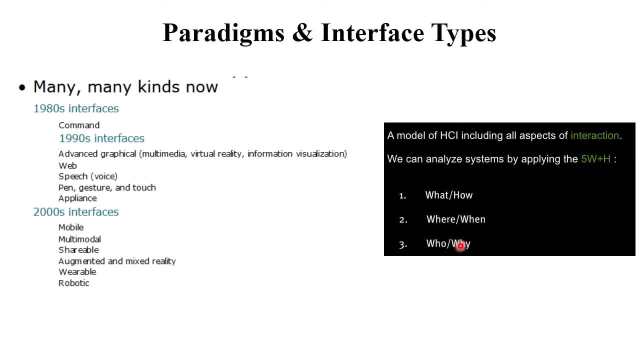 What, where, when, who and why. These are the questions. So answer of those questions means Paradigms of Interaction, Right. What technologies are developed, How these technologies are developed, Right. So these all answer of all those questions included in this paradigms of interaction Clear. Next. 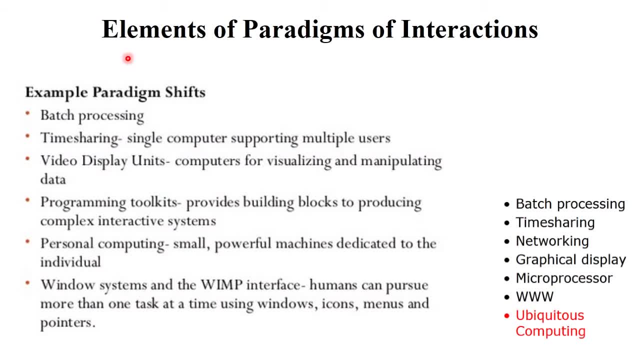 The next point is elements of paradigms of interaction. So see, there are total 7 elements of paradigms of interaction included in your syllabus, Like batch processing, time sharing, networking, graphical display, microprocessor, www, that is web page, ubiquitous computing, Right. So these are all the elements of paradigms of interaction. 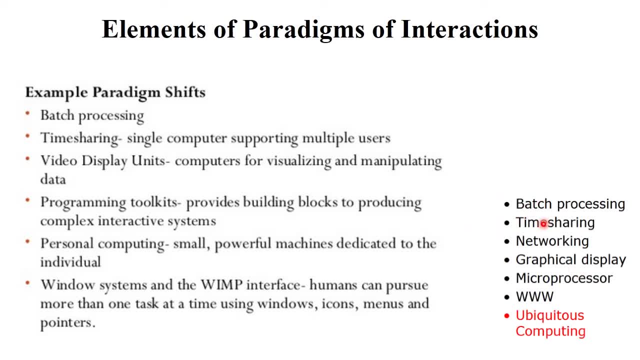 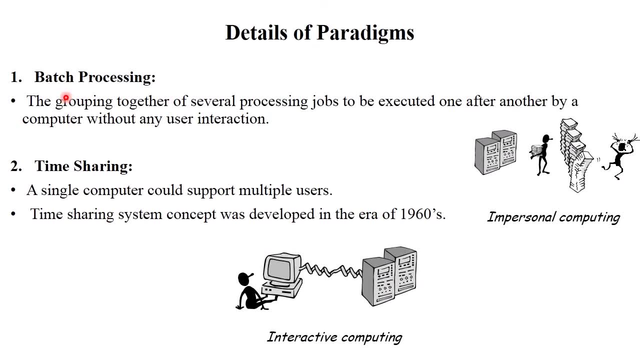 So in the next slide I will explain one by one Next. So next, details of paradigms. The first element of paradigms is batch processing. We all are familiar with operating system or system software concept. So batch processing means the grouping together of several processing job and executed one after another by a computer without any user interaction. 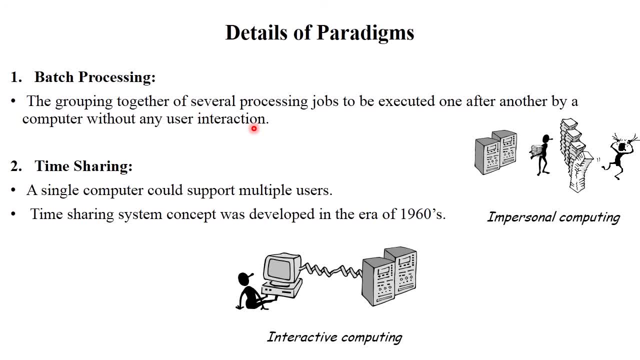 Our computer system, our mobile system, used batch processing concept. Okay, So batch processing means one by one, each and every job or task schedule, Right Without any user interaction, Which is also called as impersonal computing. Clear. The next element is time sharing. We all are familiar with time sharing operating system. A single computer could support multiple users. Time sharing system concept was developed in the era of 1960s. 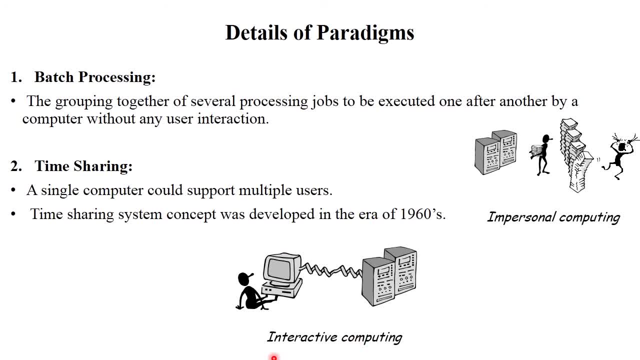 So this time sharing operating system is also called as interactive computing. This single computer could support multiple users. Many users works on the same computer at the same time, Right So this concept invented in 1960s, It's called as time sharing operating system. Clear. 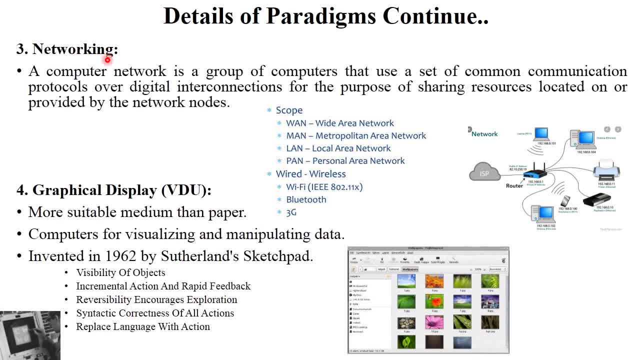 Next, The next element of paradigms is networking. Again, we will study networking A computer network. A computer network is a group of computers. It means it uses set of common communication protocols over digital interconnection for the purpose of sharing resources located and provided by the network nodes. 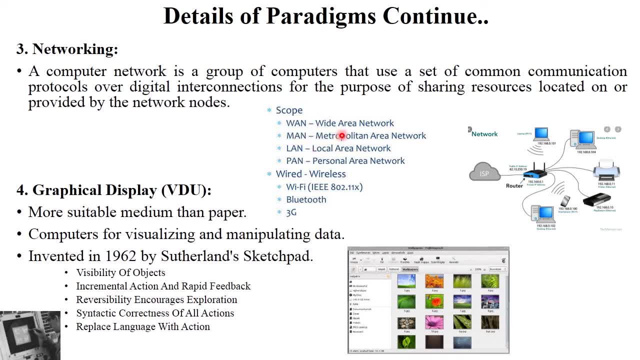 Right. There are different types of network: LAN, like wide area network, metropolitan area network, local area network, personal area network. These all kind of networks are available Clear, And also there are some wired devices or wireless devices, which includes Wi-Fi, Bluetooth, etc. 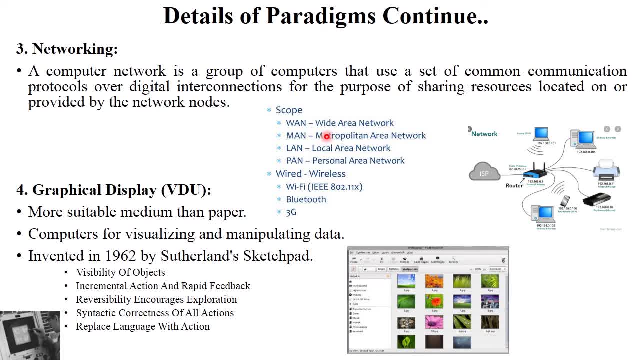 So again, these are the new inventions in networking. Different types of networks, scopes, and there are different types of features or specifications are included in networking system. Clear Next element is graphical display. So graphical display is more suitable medium than paper. 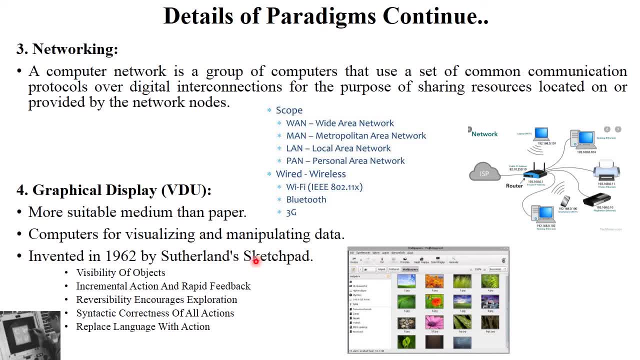 It is invented in 1962 by Sketchpad, So the name Sketchpad Right. So computers were visualizing and manipulating data by using graphical display. It is a most interactive system. like graphical system, So graphical display is useful for visibility of objects, incremental action and rapid feedback. re-vergulability encourages exploration, synthetic correctness of all actions and replace language with actions. 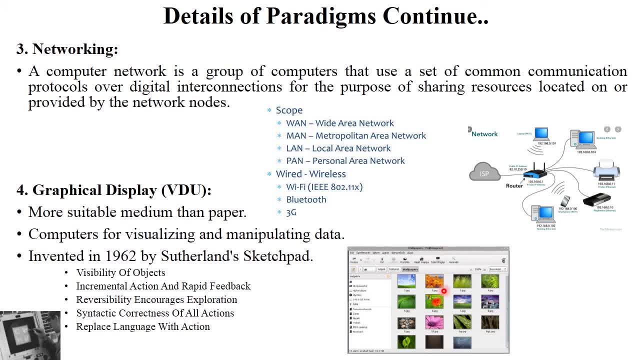 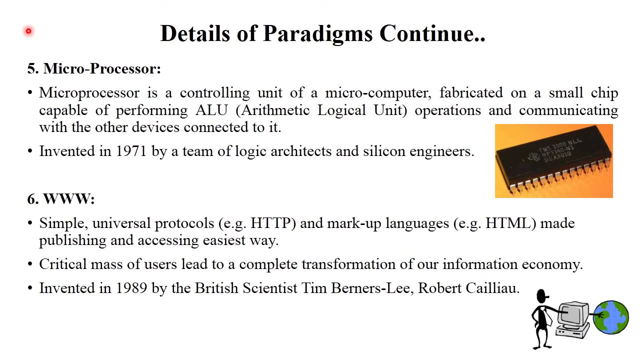 So graphical display is very easy to understand. It is a most attractive Okay. Okay. So graphical display is also called as visual display unit, That is VDU Clear Next. Now, the next elements or paradigms of interaction is microprocessor. 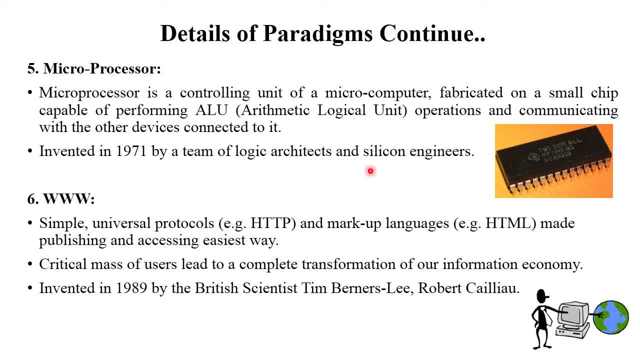 We all are familiar with microprocessor chip Right. So microprocessor is a controlling unit of microcomputer. It is a fabricated or small chip capable and performing arithmetical logical operations and communicating with the computer. It is also connected with the other device connected to it. 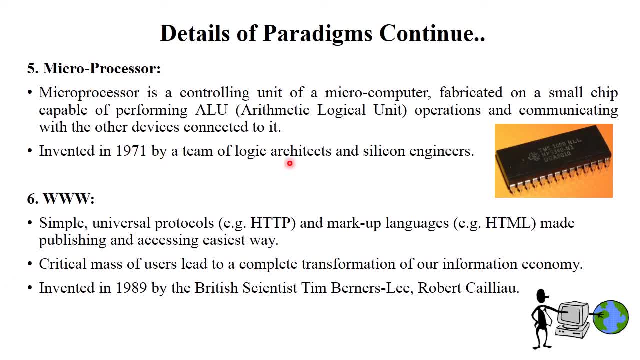 Microprocessor is invented in 1971 by team of logic architects and silicon engineers. Right And the next element of paradigms of interaction is WWW, World Wide Web. We all are familiar with this. For World Wide Web, there are different protocols like HTTP, then FTP, TCP. 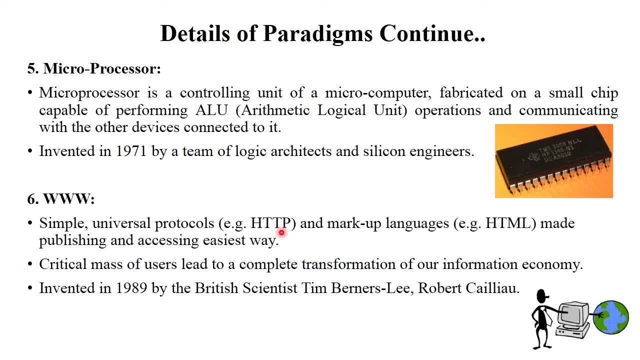 These kind of protocols are used for networking, file sharing purposes And also different types of web languages like HTML, CSS, then JavaScript and nowadays there are Python, PHP. These kind of languages are used for publishing and development of websites and accessing easiest way. 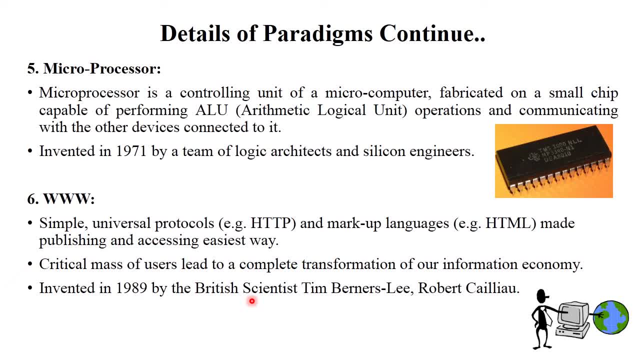 WWW, invented in 1989 by the British scientist Tim Berners-Lee and Robert Scully. Right So WWW is a complete transformation of our information. Right So WWW is a complete transformation of our information. Right So WWW is a complete transformation of our information. 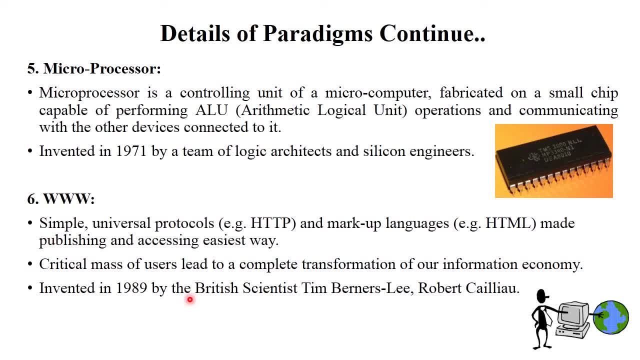